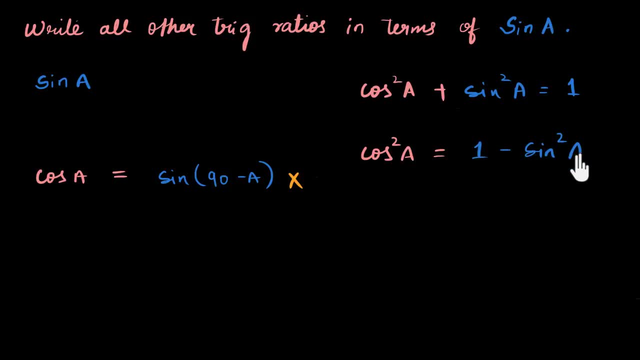 square a, subtracting sine square a on both the sides. And now then, what is cos a? Cos a is going to be, that's right. cos a is just root over, root over 1 minus sine square a. So I'm going to. 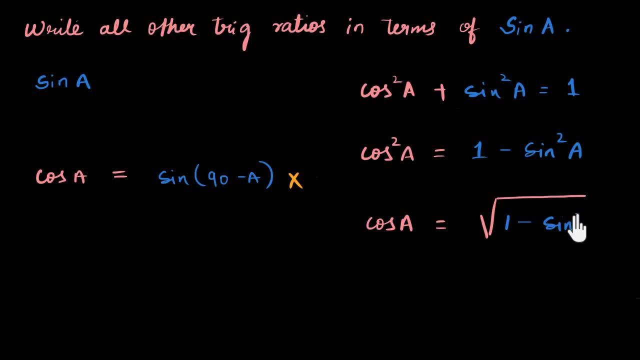 find sin square a 1 minus sine square a, And you can be happy here. or you can ask me: hey, wait a minute. if cos square a is equal to 1 minus sine square a, then isn't cos a also possibly negative? 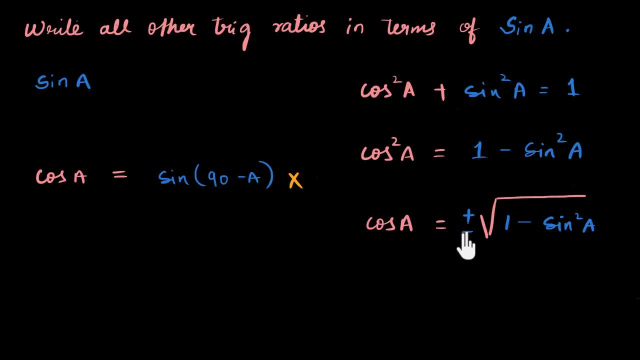 So shouldn't I put a plus or minus sign out over here? In other words, if I don't know this cos square a is, I don't know 4, then cos a could be 2, but it could also be minus 2.. So there is a. 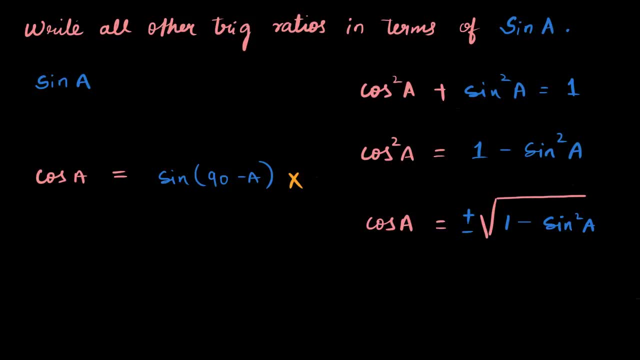 plus sign out over here. So I'm going to put a plus or minus sign out over here. So I'm going to put a plus or minus sign over here and you will be correct. But given we are in class 10, in class, 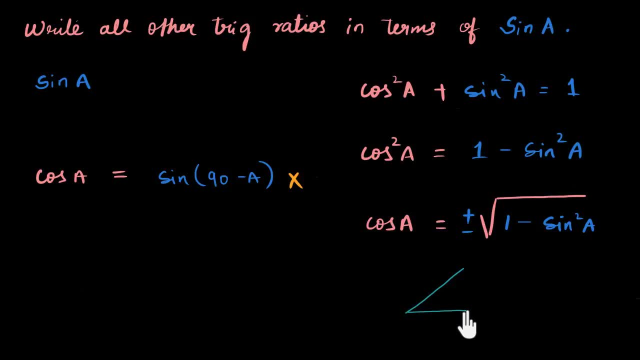 10,. cos a is basically: if you have a triangle like this, a right angle triangle, if this angle is a, then cos a is basically this length by this length. right, And this length is a positive number. This length is a positive number, So this length by this length will also be a positive. 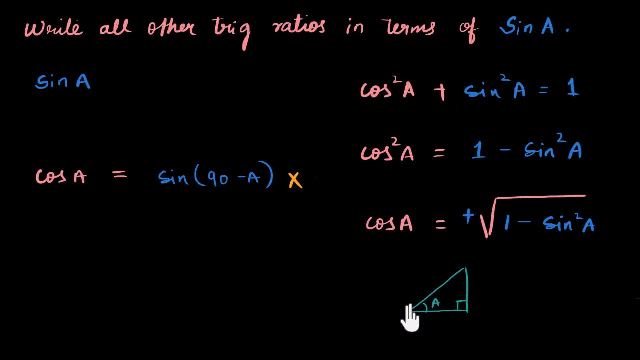 number. So but why did I say in class 10, this is cos theta or cos theta? Because if you have a cos a, does what we mean by cos a change when we grow up. It kind of does What we're dealing with. 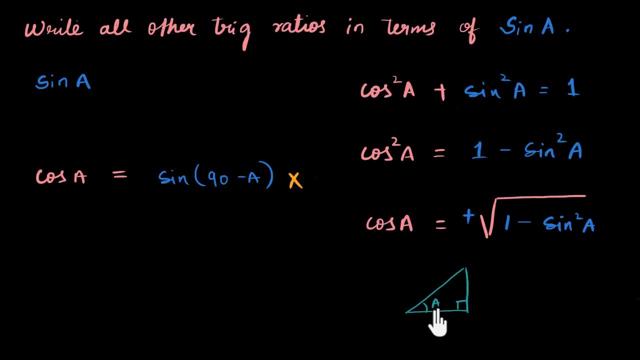 in class 10 is what I like to call the demo version of trigonometry, where cos a is this ratio of this side by this side of a triangle, which means it will always be positive, because this will be positive and this will be positive, But later, when the full version unlocks of trigonometry. 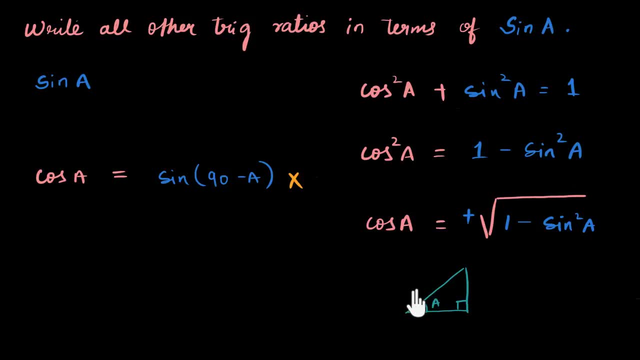 you will know that cos a can also take negative values. But as of now you don't have to worry about it because it's a ratio of lengths, It is a positive value, But later, cos sin, tan, all of them can take negative values because the way 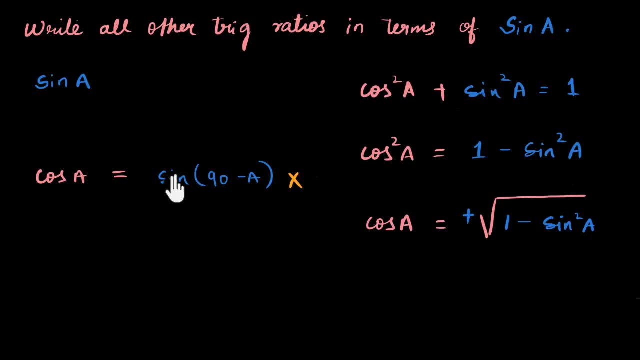 you think about them will be different. So let's update what cos of a is. Cos of a is root over 1 minus sin square a. Root over 1 minus sin square a. You'll probably use this a lot. Now let's go. 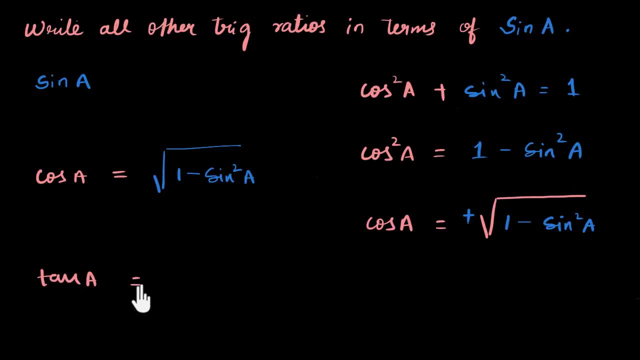 to tan a, Tan a, Because once I have cos and tan- and I already have sin- it's easy for me to find the reciprocals, because the other three are just reciprocals of these. Now, I've already used this. 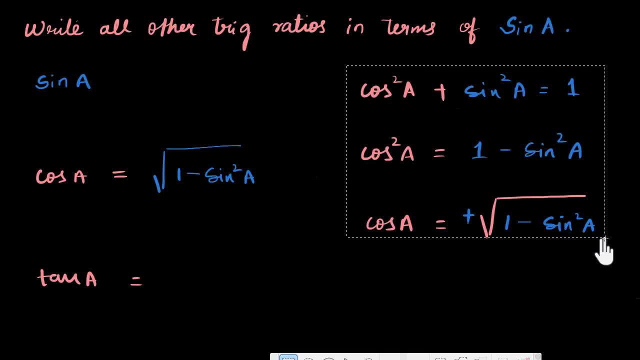 one here. I don't need this anymore. So let's get rid of this to make some space Bye-bye. So tan of a. So I know already an identity that connects tan and sin and that's tan a equals. 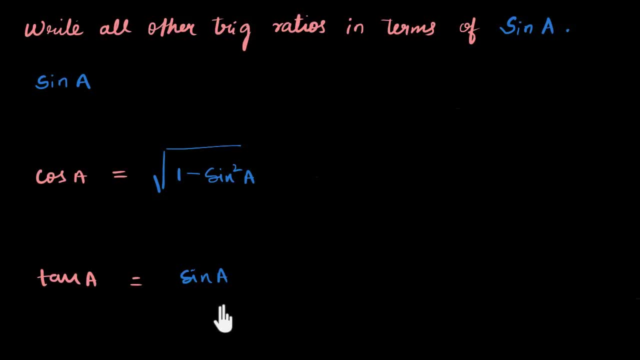 sin a by cos a. That itself is an identity, And I know that I already have a sin a here. I have to now find cos a in terms of sin a, but I already did that hard work, So I can just use it. 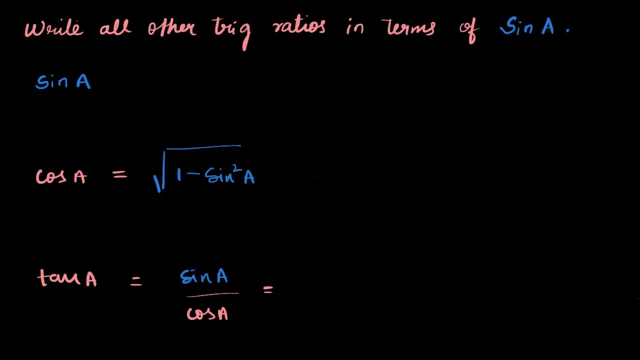 So if I use that, then I'll get equals sin of a by root over 1, minus sin square a, Sin square a. And that's it I'm done. because the other three? Let's draw a nice line over here. The other three. 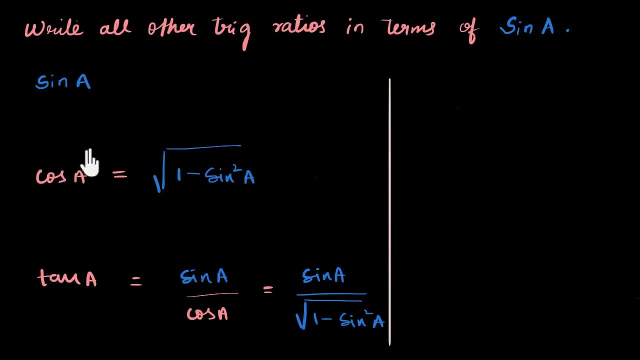 That's not a nice line. A nice line over here. The other three are just reciprocals, So the easiest of this is actually cosecant a, Cosecant a, Because that's just equal to 1 by sin a. 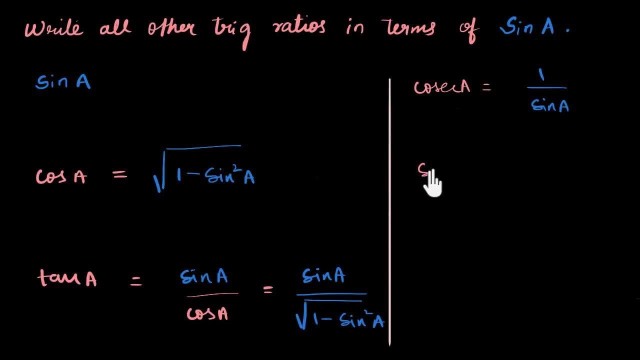 1 by sin a. Then we have secant a, which is just 1 by cos a, And I can just write 1 by this now, because I already did that hard work: Root of 1 minus sin square a, And the same story over here. 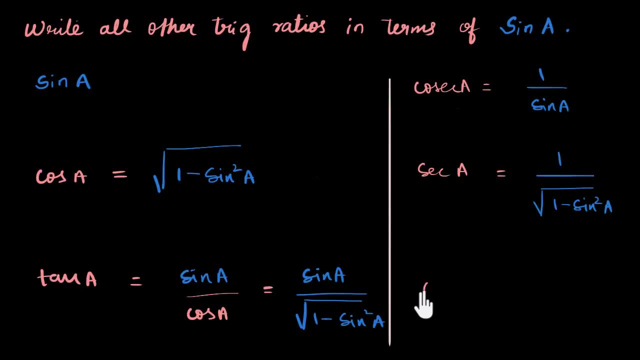 for tan a. The reciprocal of tan a is cot of a, And that's going to be equal to the reciprocal of this, which is root over 1 minus sin square a Divided by sin a. So notice that whenever you have to find other trigonometric ratios you probably have to find 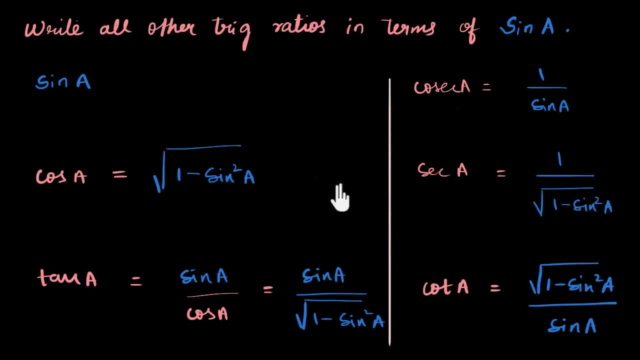 2. And that's it, because the others will be reciprocals. Even though it seems like you have to find 5 other ratios, you only have to find 2..